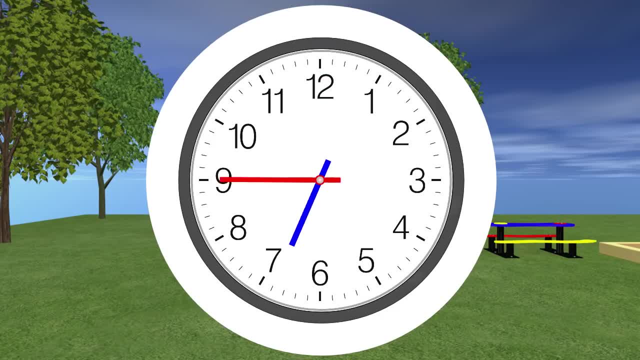 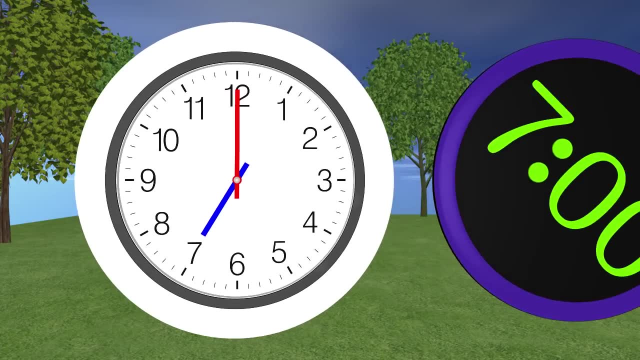 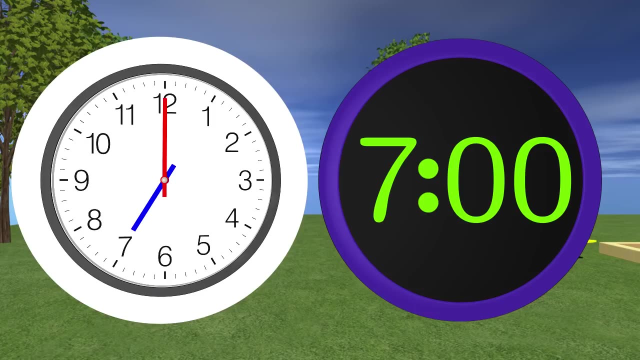 minute hand points straight up because it is on the hour. What time is it? right now It is 7 o'clock. Great job. again On the right side I have a digital clock which, as we learned before, shows time, but only using numbers. Both of these clocks show 7 o'clock. The digital clock shows 7 for the 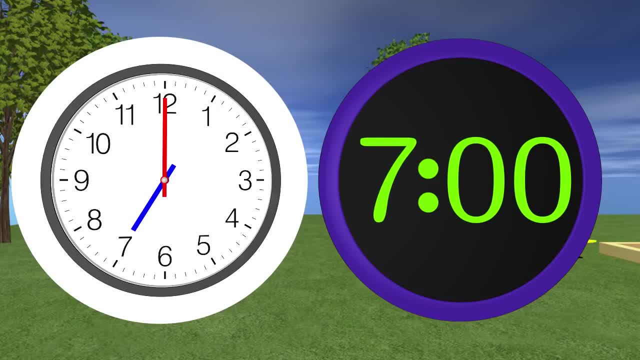 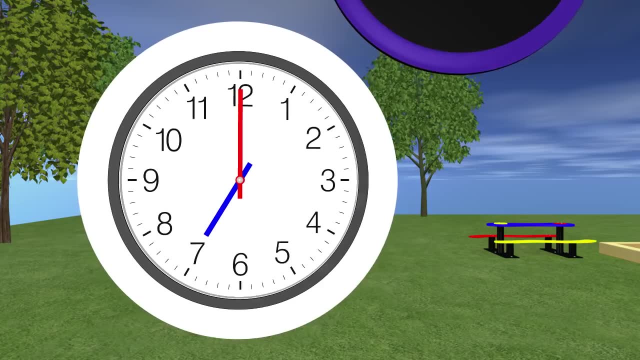 hour and the two zeros show the minutes. Right now the hour is 7 and the minutes are zero, so we say 7 o'clock. This time stuff is really cool guys. Now that we know what o'clock means, it is time to learn about half hours, so I can know. 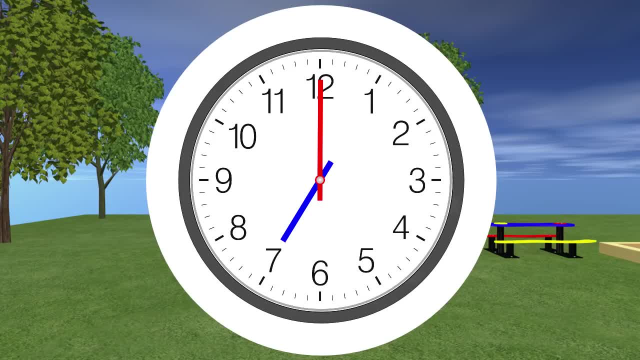 when to go to my basketball game. Right now, the time on the clock is 7 o'clock. We say 7 o'clock when the minute hand points straight up because it is on the hour. What time is it right now? Right now the time is 7 o'clock. but watch this: The minute hand is moving around the 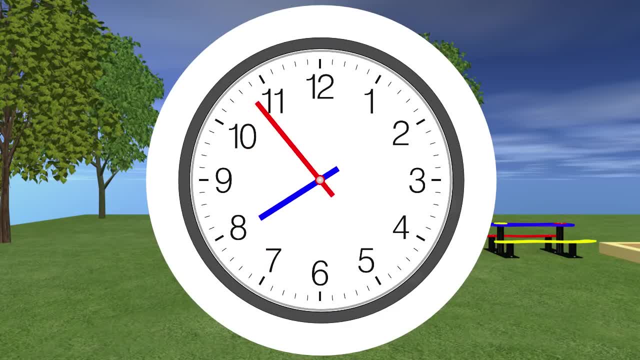 clock, but you will also notice that the hour hand is moving as well. While the minute hand went all the way around the clock, the hour hand moved from the 7 to the 8. That means one hour went by For the minute hand to go all the way around the clock. it has to go. 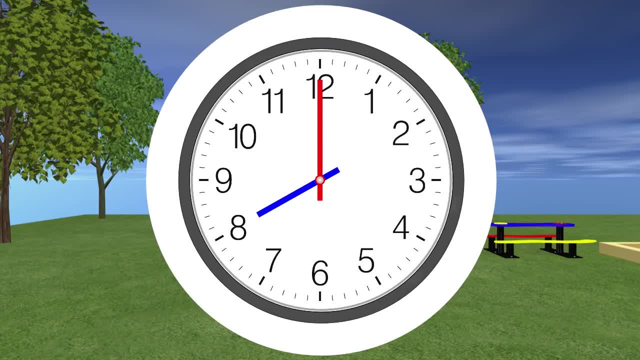 around 60 minutes. So 60 minutes is how long it takes for the minute hand to go around the clock. once Now I am going to take the minute hand halfway around the clock. Where would the minute hand point to if it just went halfway around the clock? Let's see, Mr Clock, would you please? 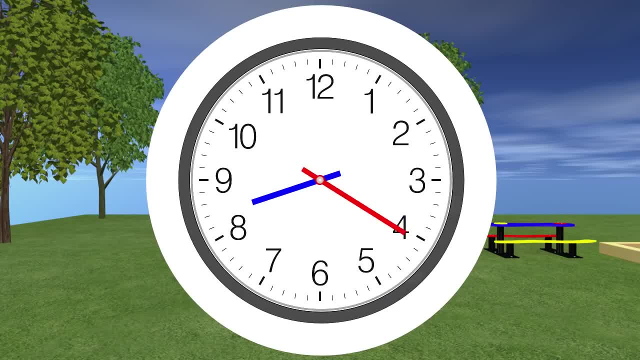 move your minute hand halfway around the clock. Now we can see that the minute hand has gone halfway around the clock and has stopped at the 6. The small numbers on this clock are the minutes The minute stopped. at what number The minute hand is pointing to the 30 minute. 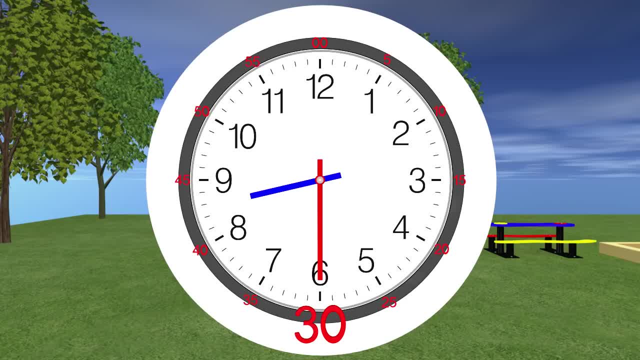 hand to the 30-minute mark. Halfway around the clock is 30 minutes. Great job, kids. The hour hand is in between the 8 and the 9.. While the minute hand went halfway around the clock, the hour hand only moved halfway between the 8 and the 9.. This is confusing. 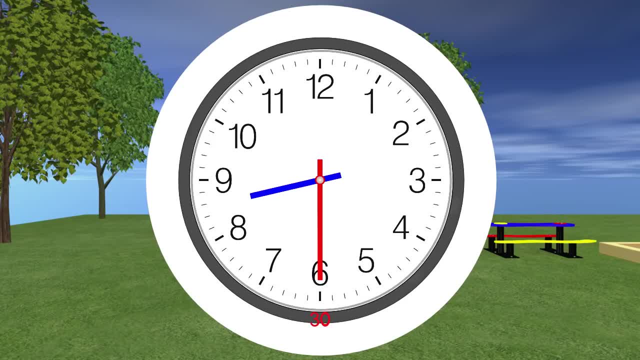 because I do not know the hour. Do you think the hour is 8 or 9?? The hour is still 8, even though it is past the 8.. When the hour hand points right at a number, it starts the hour. It stays that hour until it reaches the next number. 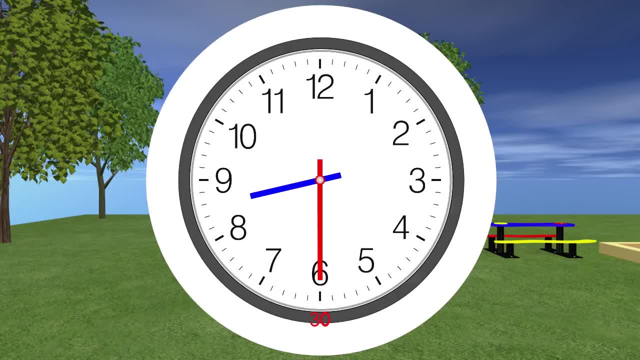 Right now the hour hand is past the 8, halfway and we see that the minute hand is pointing to the 30. We can say that the time is half past 8 o'clock. This happens to be the time that my school starts in the morning. My parents said that school starts at half past 8, and. 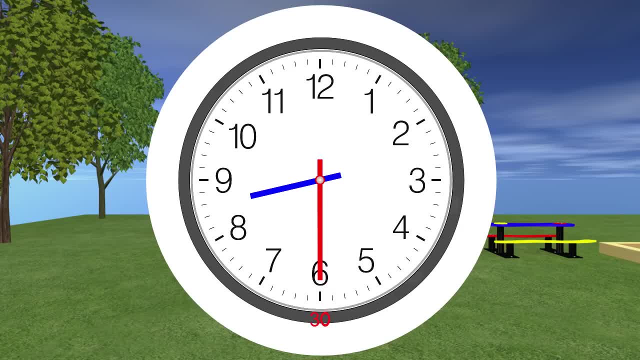 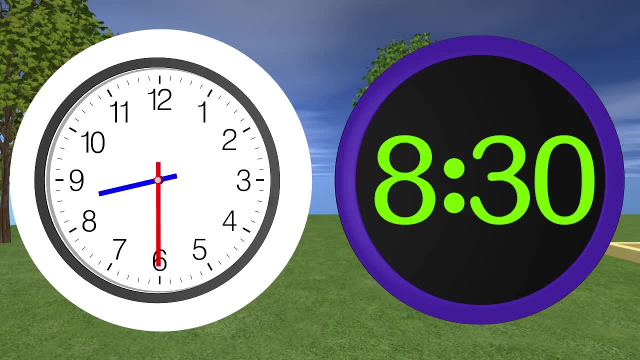 now I know what that means: 8.30!. Wow, this time stuff is awesome. We have two clocks here, the analog clock on the left and the digital clock on the right. The digital clock shows 8.30, and the analog clock shows 8.30 as well. The 8 shows the. 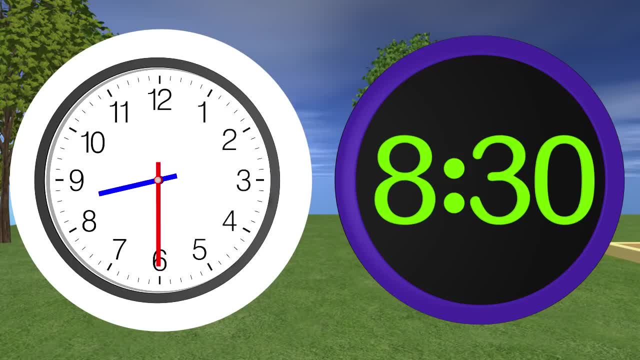 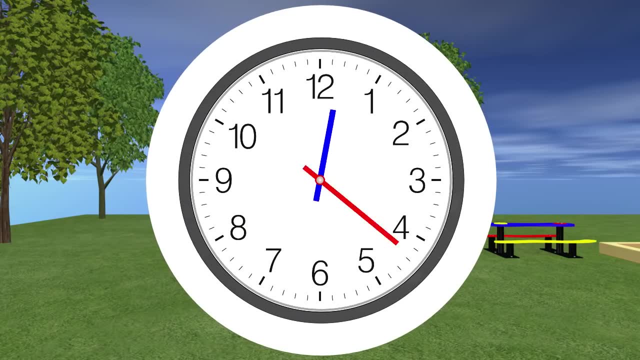 hour and the 30 shows the minutes that have passed. If we were write the time, we would write it, just like the digital clock shows. Can you tell me what time it is now? The time is 12.30. we could say it is half past 12.. Great job, kids. we can see that a half hour or 30 minutes. 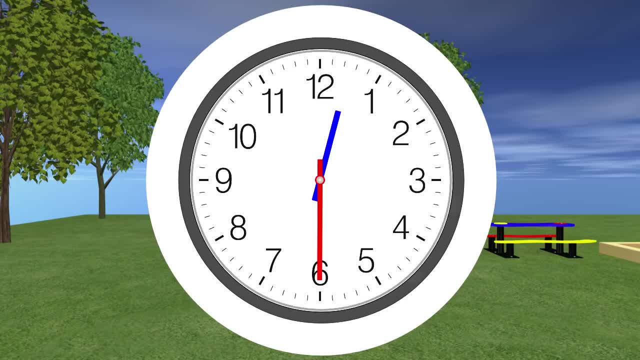 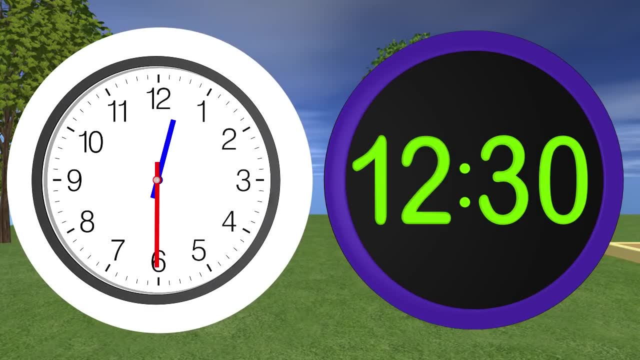 have passed since 12 o'clock. If we wanted to write this time, what would it look like? You would write it like you see it on this digital clock: 12 is the hour on the left and 30 minutes is on the right. The time is 12.30 or half past 12.. 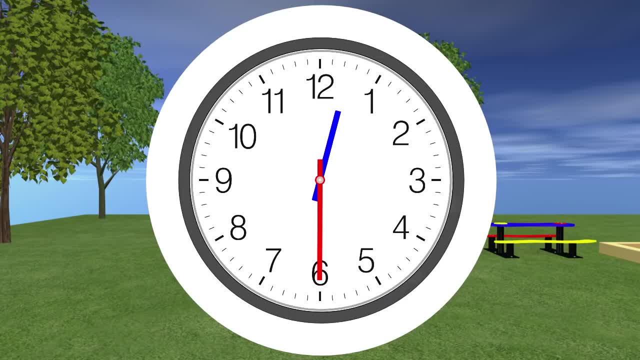 Now that we have learned a lot, can you help me figure out when my basketball game starts? They told me it starts at half past 3.. Is this half past 3?? No, this is not half past 3.. This is half past 2 o'clock. 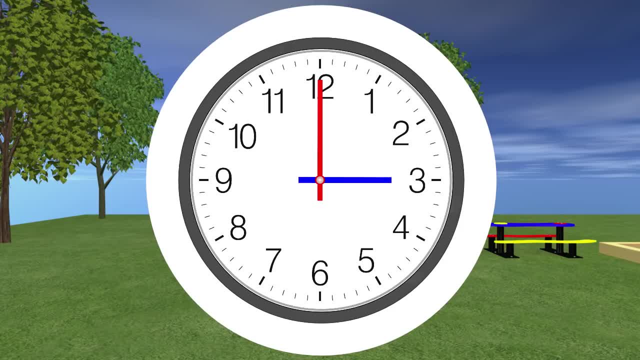 How about now? Is this half past 3?? No, this is still not half past 3.. What time is this showing? It is showing 3 o'clock. How many more minutes do I have to move the minute hand to get to?